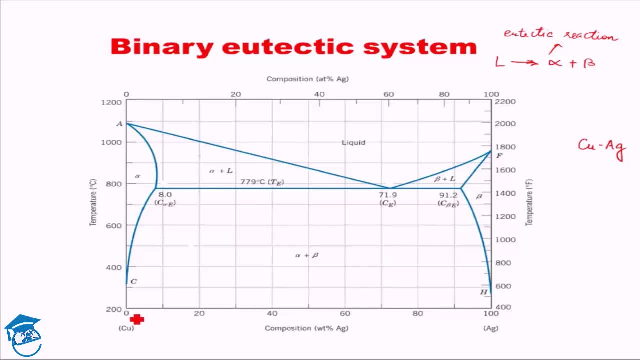 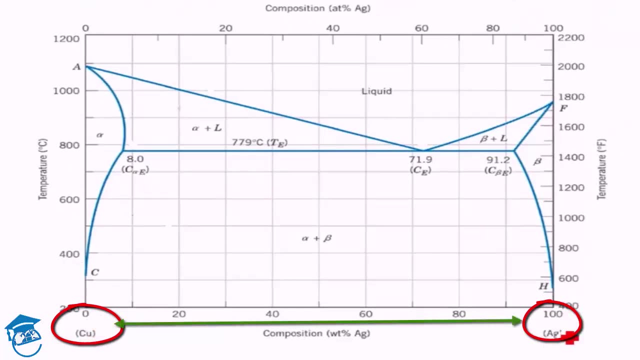 this copper silver system. Here the plot is 100% copper or 0% silver, 100% silver or 0% copper. So this is basically percentage of silver, increasing percentage of silver in the x-axis. The y-axis is the temperature. Here we have used degree Celsius and this: 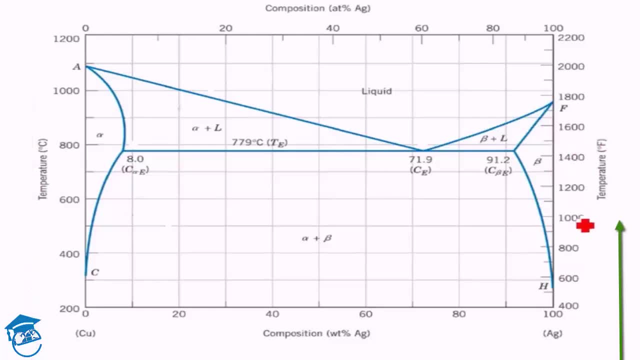 axis is degree Fahrenheit. Now there are certain differences here when compared to the isomorphous system. In the isomorphous system you had complete solubility in the liquid and the solid phase. Here we don't have that. There is complete solubility in the liquid, That is to say that the liquid exists as a single. 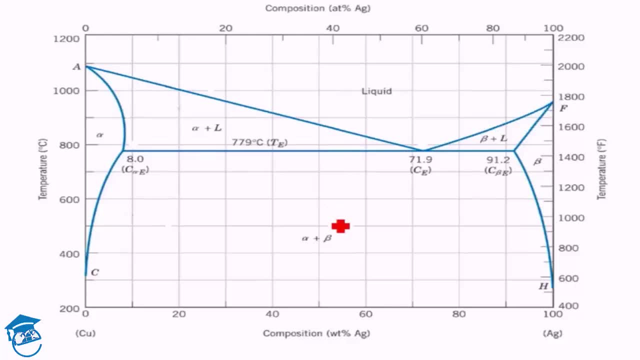 phase, but in the solid state we have two different phases coexisting, So percent solubility does not exist in the solid state. Thereby this is not an isomorphous system. Now we know that this is the liquidus line, similar to LIQUI liquidus line. This is solidus. 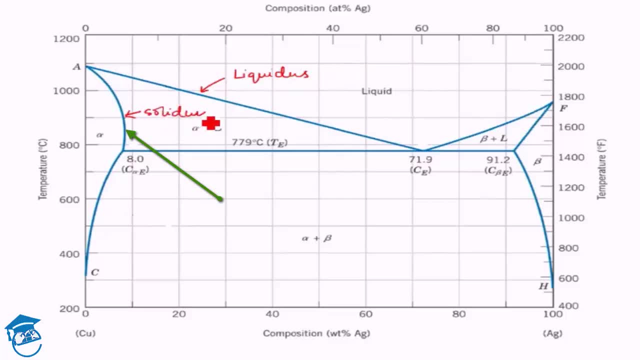 line. But here we have an additional line over here, This particular line, This particular line which is separating the single phase solid to double phase solid. This is known as the solvus line. Similarly, this is also the solvus line, This is the liquidus line and this is. 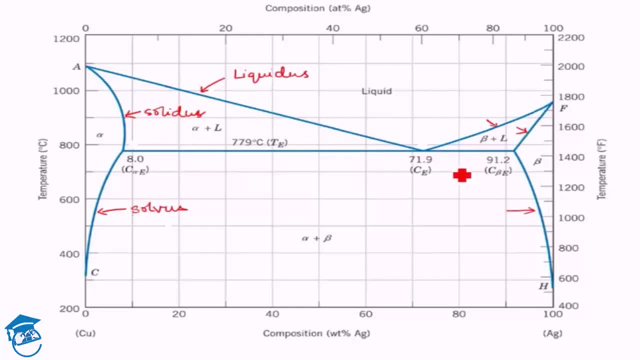 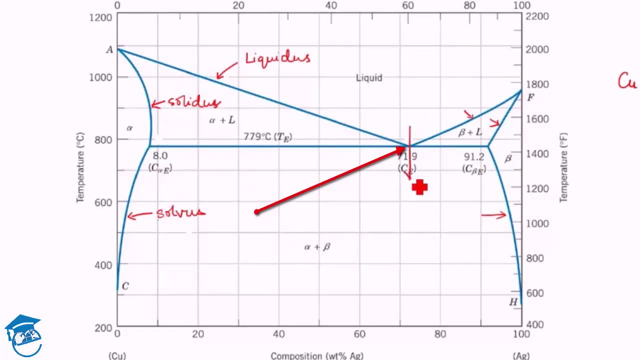 the solidus line. ok, With this in background, let us see where exactly is the eutectic reaction taking place. The eutectic reaction is taking place at this location. exactly What is happening is: here is 100% liquid, there is no other phase, and here we have two phases simultaneously occurring. 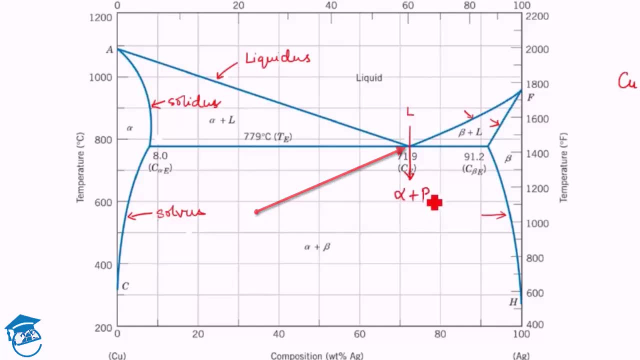 out of the liquid alpha and beta. Okay, So if you examine the eutectic phase diagram shown here, what you see is that we have one phase is the liquid phase, Then we have one phase, the alpha, and one phase, the beta phase. Alpha phase is rich in copper because it is. 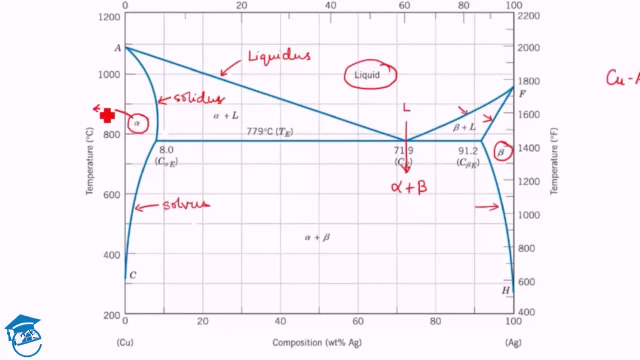 at the copper end. So this is copper rich. Beta is silver rich. Okay, Because it is at the silver end. Now these two ends are the terminal ends, Okay, Thereby this is also known as terminal solid solutions, these two, Because these are solid solutions. 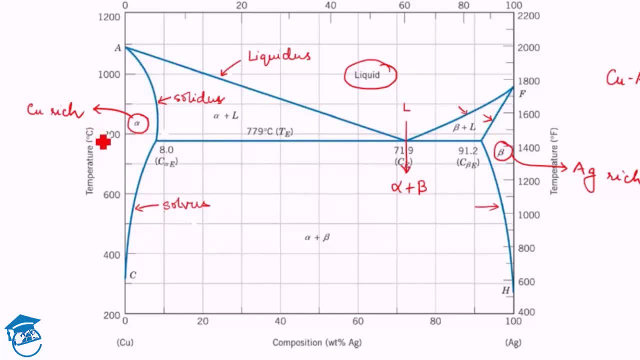 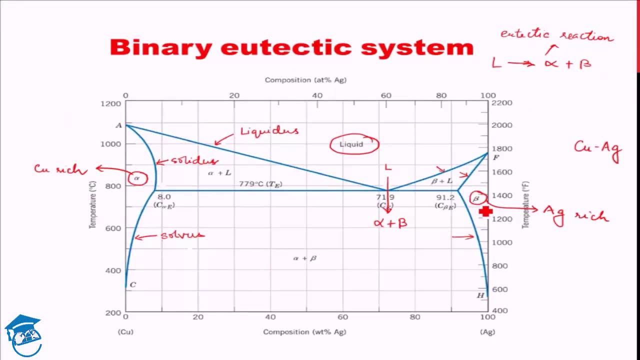 Mind you, though, this is copper rich, but there it is not pure copper. It has silver along with copper, and beta has copper as a solute in silver matrix. Fine, Now let us see several different compositions and see what exactly is happening at different composition. 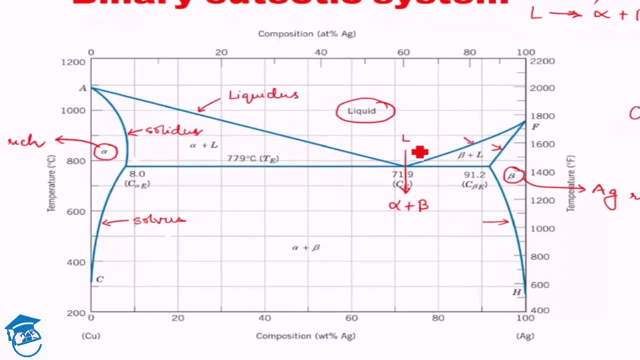 The point of our interest will be eutectic reaction, That is, this region. You see that the conversion of liquid to two solid simultaneously is called eutectic reaction. So that means that the conversion of liquid to two solid simultaneously is called eutectic reaction. 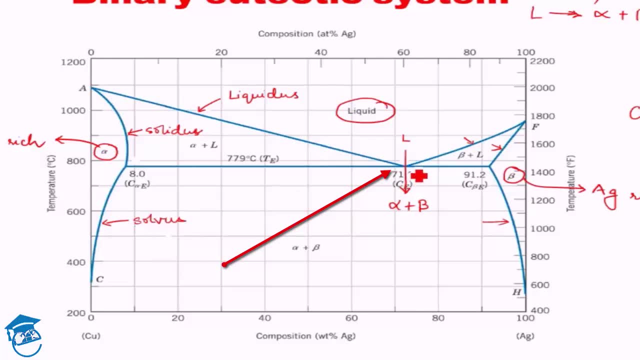 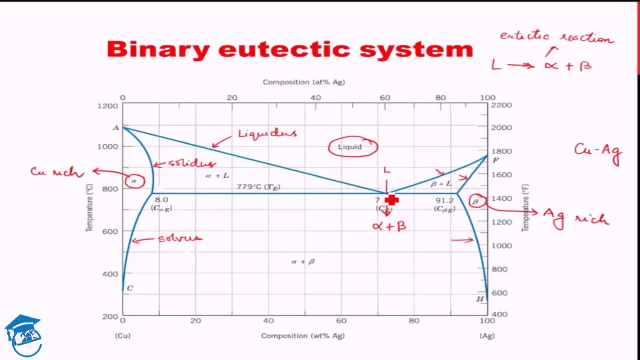 So that means that the conversion of liquid to two solid simultaneously is taking place only at one point. It's exactly at this point that that reaction is taking place. Any other location you go, this reaction won't take place. Let's assume we are over here In this. 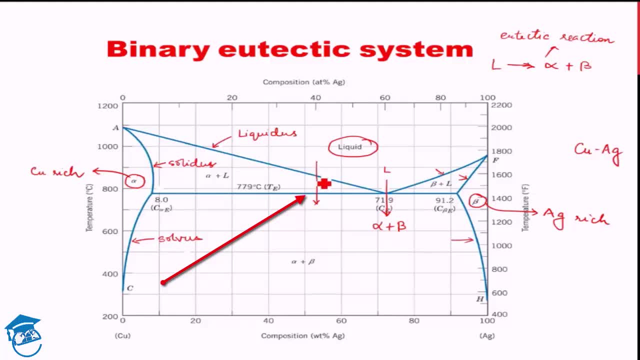 line. what will happen Over here? liquid is getting converted to liquid plus alpha, So both the solid states are not forming simultaneously. The second solid state will form only after the temperature reaches this region, Right? Similarly, if we go this way here, we form. 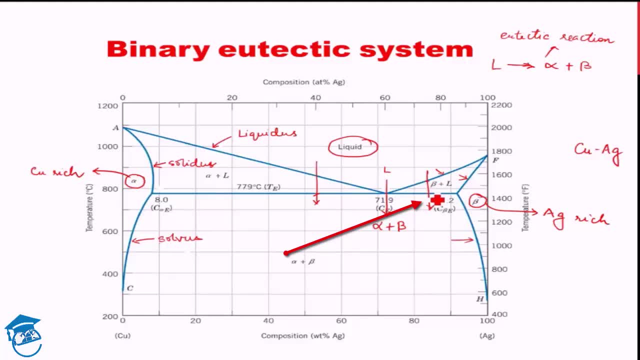 beta, but there is no alpha in this region. Alpha is formed only after we reach this temperature. If we go via any other way, actually if we go via this way- we have beta plus liquid. here no alpha And here there is only beta. All the liquid is converting to beta Now. 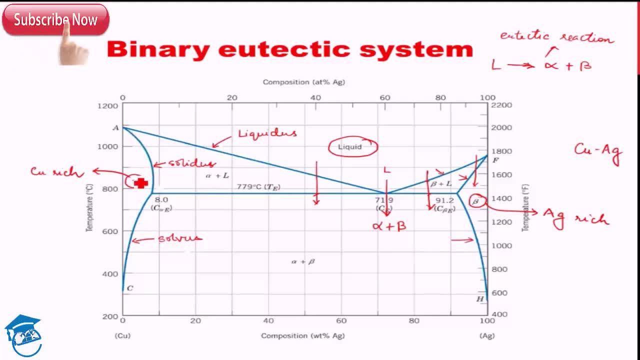 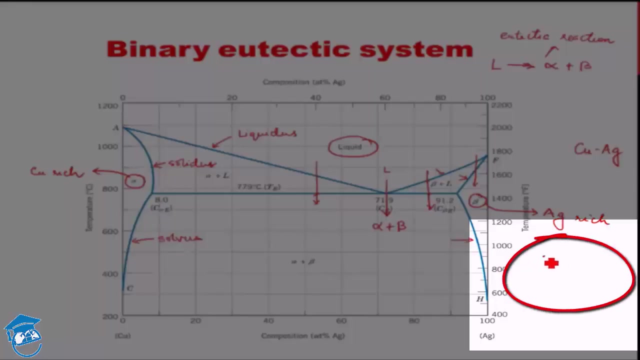 we have a parallel scenario is happening over here. So what we see is there is the possibility of eutectic reaction at a given temperature, at a given composition only. What is the combination of temperature and composition For this case? for the copper silver case, we have the eutectic. 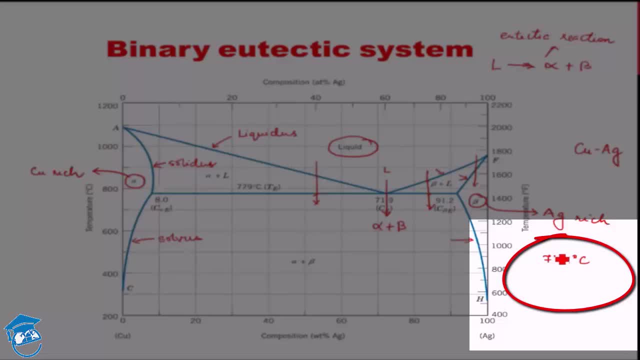 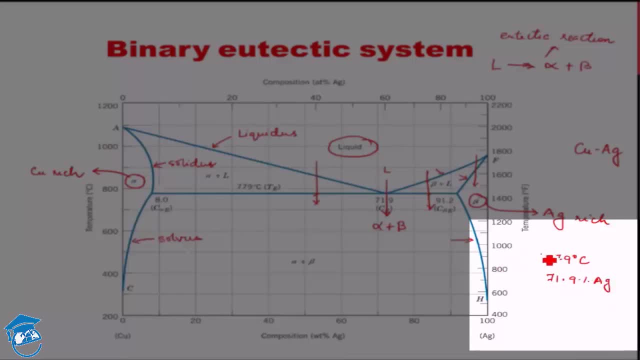 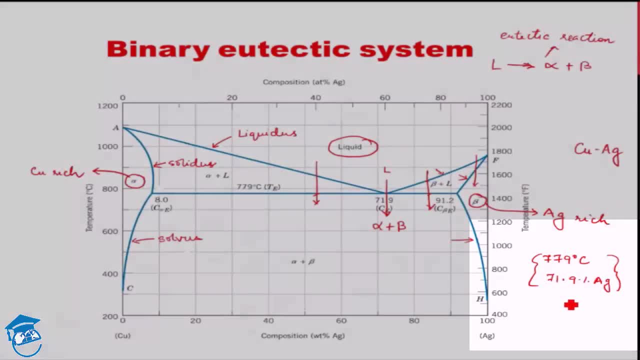 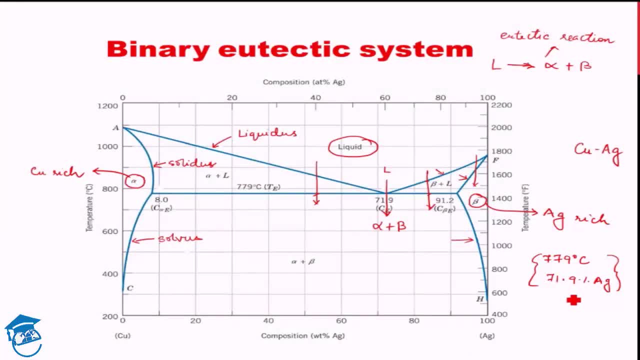 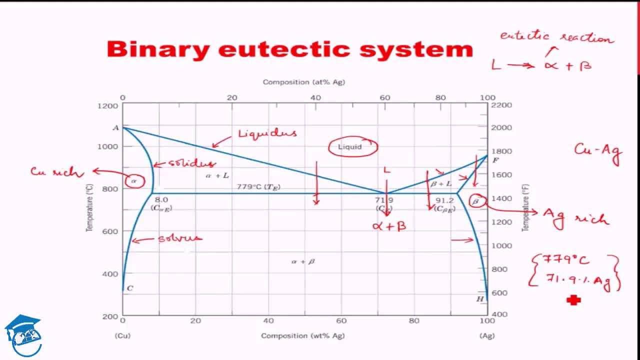 thereby this type of reaction, which takes place at only one singular point, are known as invariant reactions. they are, they fall under the category of reactions called invariant reactions. eutectic reaction is one kind of invariant reaction. okay, and we'll see later that such type of reaction 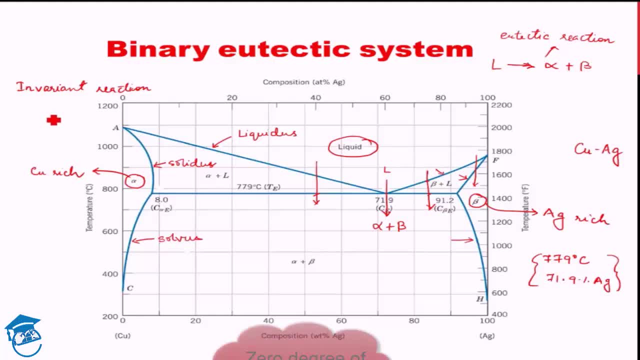 have zero degrees of freedom, that is, you do not have any choice on the parameters at which that reaction is present, will take place. it's a fixed conditioned reaction, so it has zero degrees of freedom. we'll see that later. okay, so the fundamental is liquid converting to two. 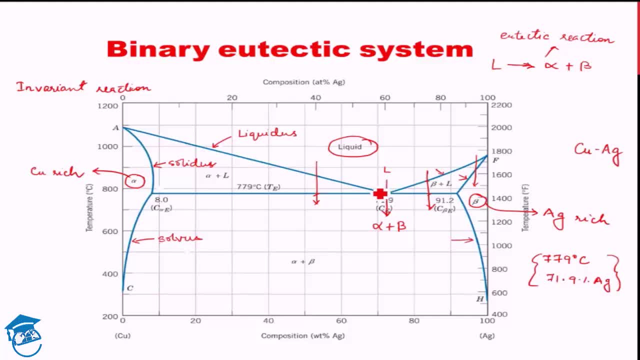 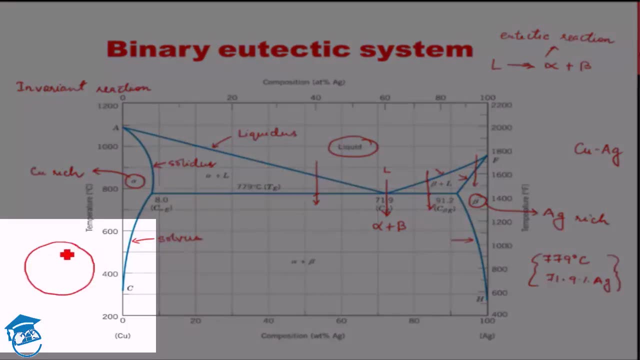 solids simultaneously. now how exactly will that happen? how exactly will a single liquid form two solids? what happens is- let me try to draw here. we are taking a sample of the liquid. first nucleus will grow. suppose we got a nucleus. then what will happen is that this nucleus which has grown 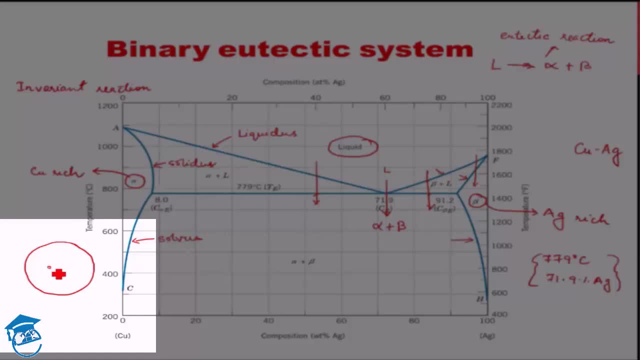 will simultaneously lead to growth of two different solid phases- alpha phase and beta phase- and the growth will be seen to be in lamellar form. so there will be a alpha lamellae, and between two alpha lamellae there will be a beta lamellae, so you will have a lamellar structure. 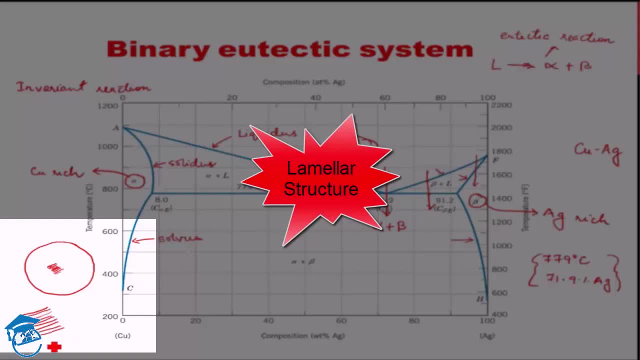 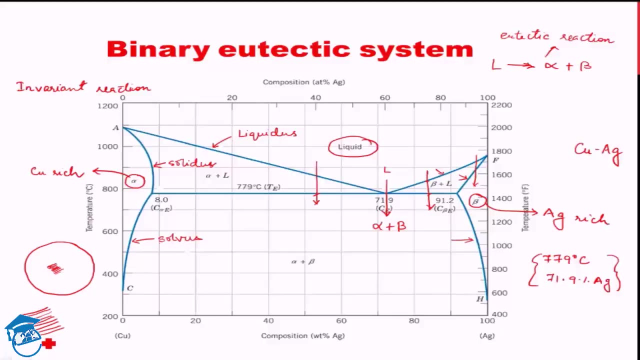 this is trademark eutectic reaction, a lamellar structure. later we'll see that a eutectic reaction takes place in the case of iron carbon diagram 2, which is a very, very important, crucial diagram in steel making. so the growth of the solid in eutectic reaction or the solid formation in eutectic 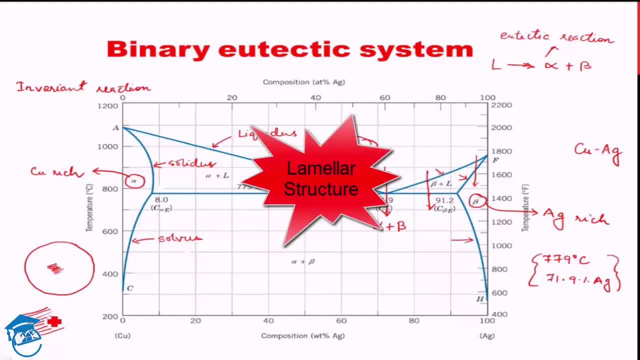 reaction leads to lamellar structure, because both the solids need to form simultaneously from the liquid. fine, now what will be the composition of the solids form? suppose we are at this condition: we solidify the liquid. we, let's suppose, are at this temperature. then what will be the composition of? 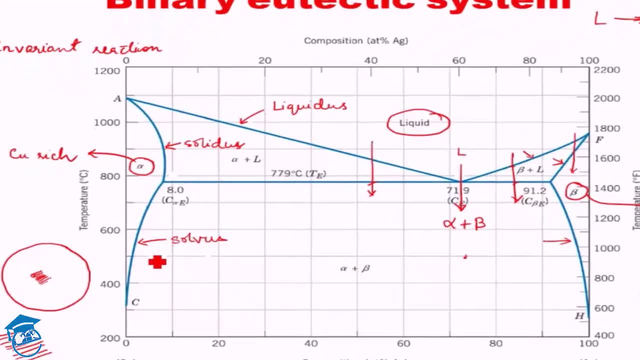 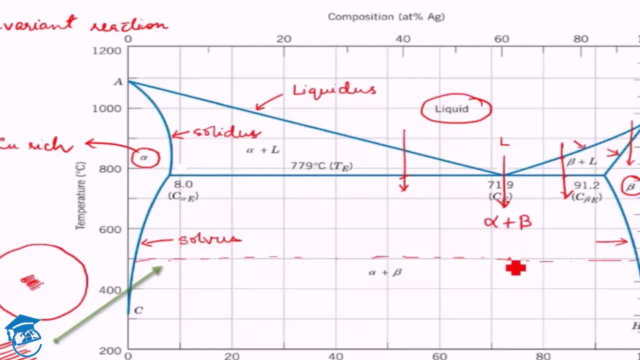 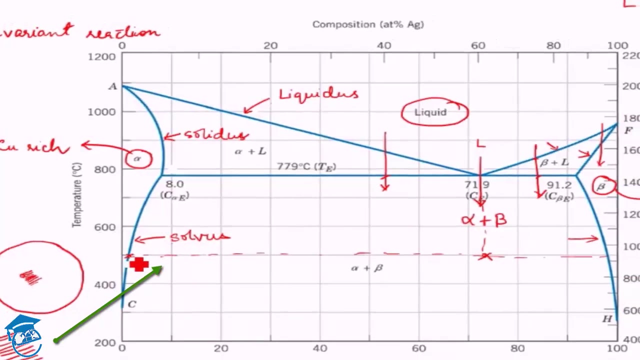 the solids. the composition of the solid can be found out by the, as i said, the isothermal line. if we draw over here, isothermal line will give us the alpha will be of this composition and the beta will be of this composition. so the alpha will be somewhere. 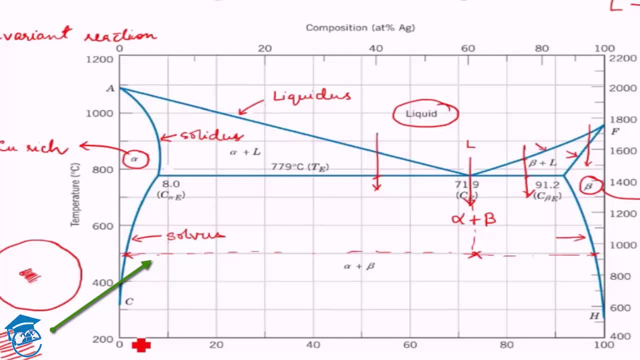 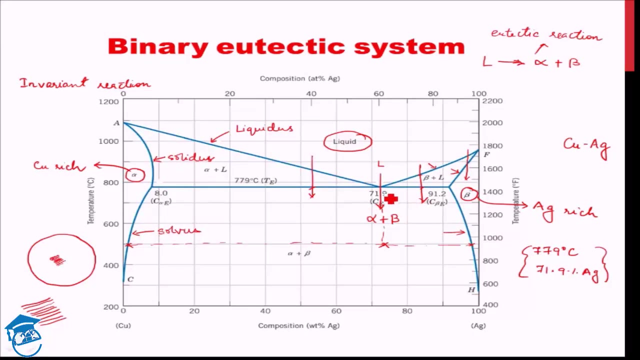 around, i guess, two percent silver and the beta will be around 98 percent silver or something fine. so, reading from the phase diagram, we can see what is happening is that as we come down in temperature, the alpha is losing its solute. the solute concentration is decreasing along this line. 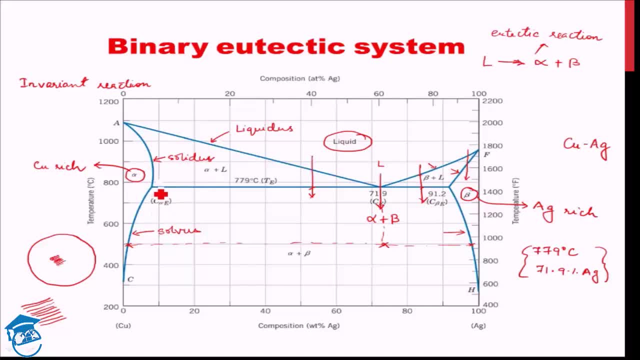 at high temperature we have larger amount of solute- almost 0 percent silver at around 750 degree celsius and that comes down to almost 0 percent at 400 degree celsius. so this also gives you an idea that with increase in temperature the solubility increases. 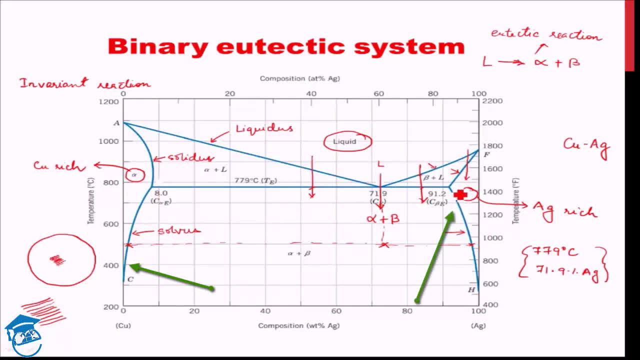 similarly over here. beta. the amount of solute is large and approximately equal to 8 percent at 779 degree celsius, whereas it comes down to around one percent at 400 degree celsius. right this temperature. it's a fixed temperature: 779 degree celsius. this is the temperature at which the eutectic 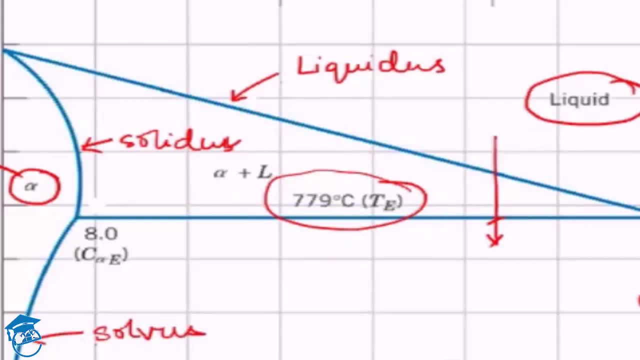 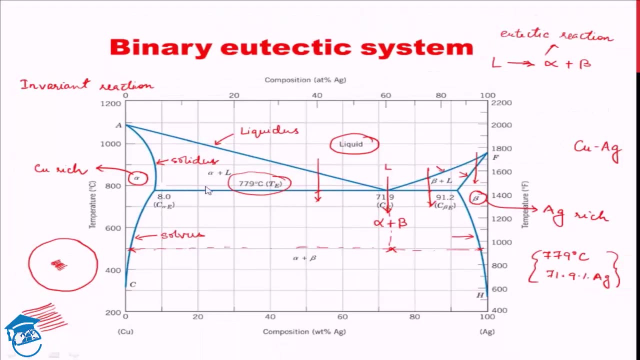 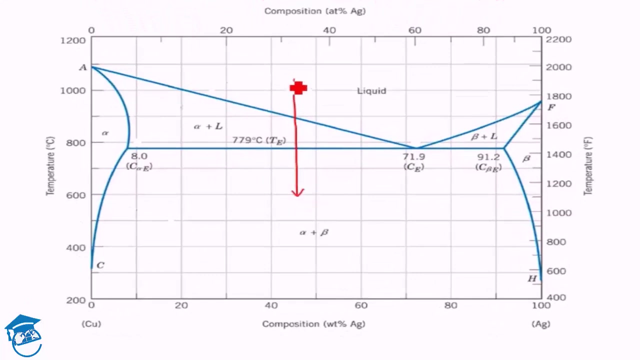 reaction takes place. now let us see what will happen if we cool the liquid at any temperature other than the eutectic temperature. what will be the result of that? let's say, we cool the liquid at this temperature, rather, we cool the liquid of this composition. 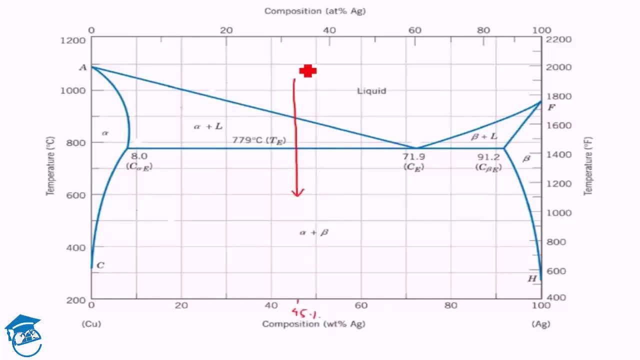 let's assume this is 45 percent silver. what will happen is it's 100 percent liquid here. as soon as it hits the liquidus line it will start to form alpha nucleus and alpha phase within the liquid. so somewhere around here what we'll have is liquid having a concentration of this. 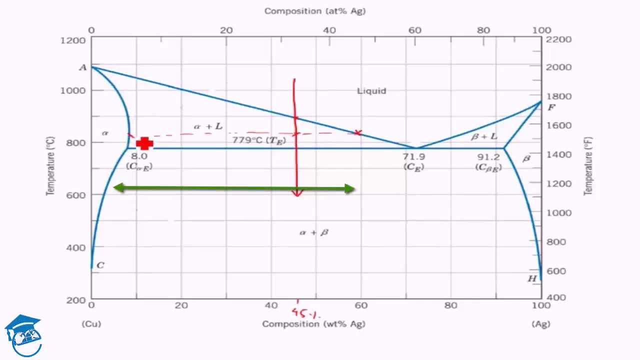 or a composition, this and alpha having composition this right. when we are about to reach this location, the process will capsize between the eutectic temperature. What will happen is that now we will have alpha of composition- this, this composition- and liquid of eutectic composition. You see, because the liquid composition 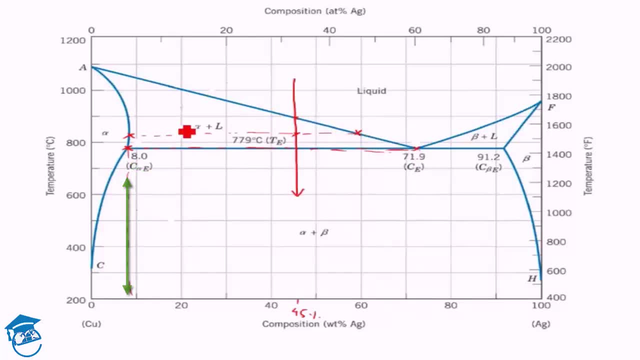 which you are getting is along the liquidus line and solid is along the solidus line. So the liquid which is left now will have a composition, eutectic composition, which is 71.9% silver. Okay, There, by once we hit the eutectic temperature, we will have liquid. 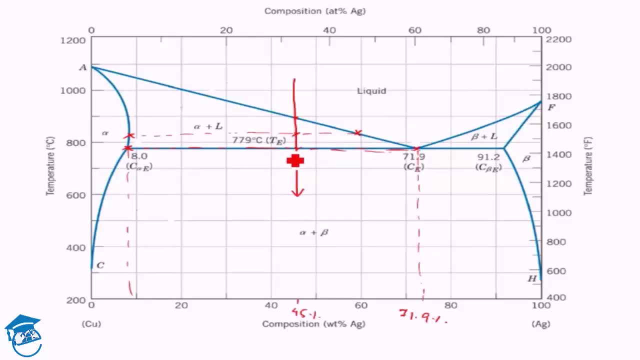 of eutectic composition and how much liquid will be left. that will be found out by the liver rule. So we will have this distance. Okay, Upon this distance, That much amount, that much fraction of liquid of eutectic composition. 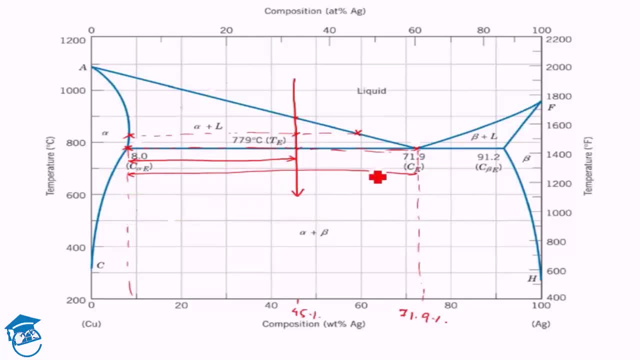 will still be left Right Now, the liquid which we have, since it is again of eutectic composition and since we are at eutectic temperature, the remaining liquid, that is, this upon this, that fraction of liquid, will undergo eutectic composition. 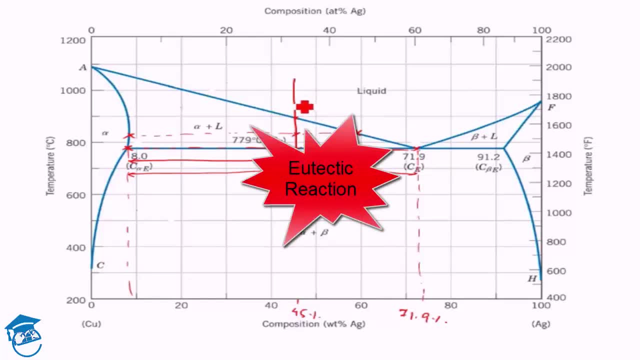 Okay, So this is the eutectic reaction. now, Even though the initial liquid was completely different composition- It was 45%- But as soon as we hit the eutectic temperature, the remaining liquid we got was of eutectic composition. See, so the interesting thing over here is: 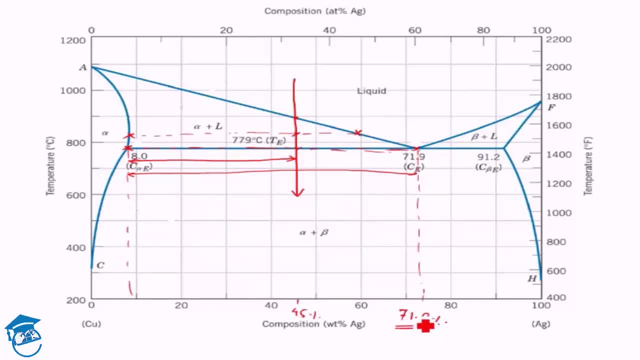 it does not matter whether the starting liquid is of eutectic composition or not. If the process is a equilibrium process, That is, we provide sufficient amount for diffusion, Then the final amount of liquid which will be left at eutectic temperature when we reach eutectic temperature will be: 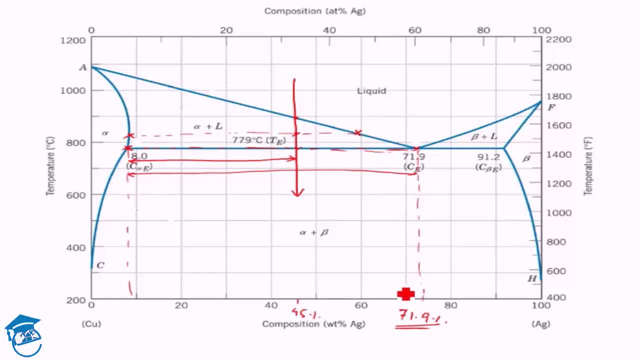 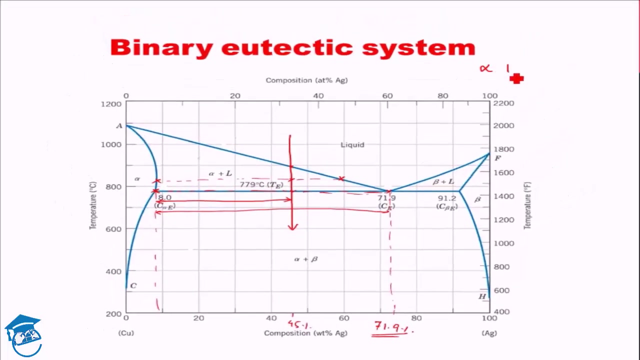 of eutectic composition, no doubt, And that has to undergo eutectic reaction. Okay, So the leftover liquid will undergo eutectic reaction and we already have some alpha over here. So what will happen is we at this region will have alpha plus liquid, which is again. 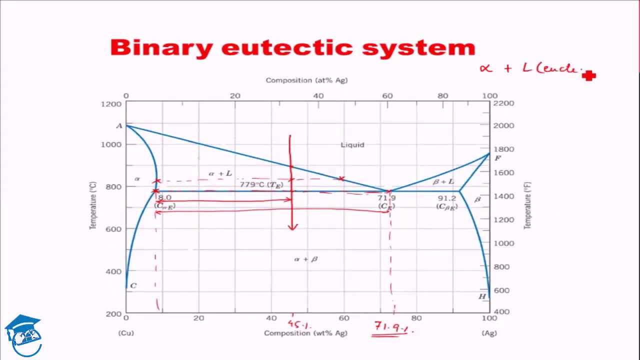 eutectic, and this eutectic will again undergo reaction on further lowering of temperature, giving alpha plus beta. This alpha is sometimes termed as pre-eutectic alpha And this is formed in lamellar form. This is not part of the lamellar structure. 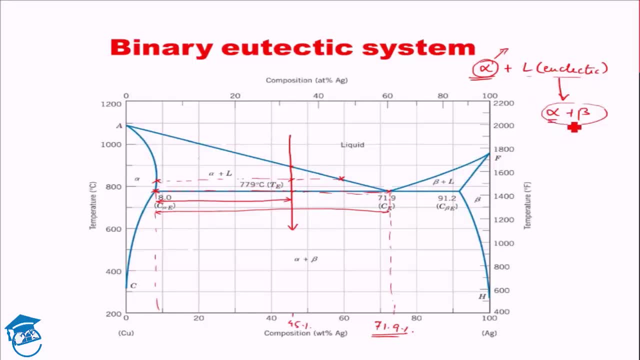 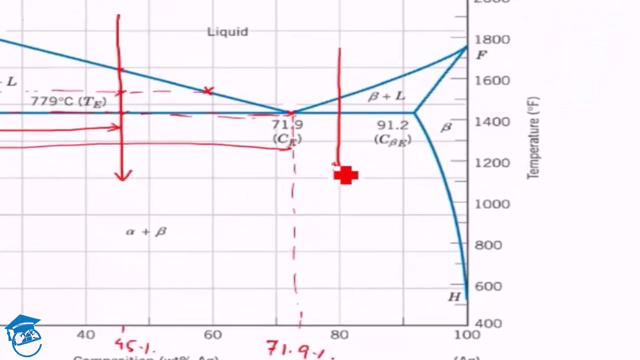 These are independent grains, but this alpha over here will be lamellar structure. Similarly, if we underwent the, undertook a composition on the opposite end, let's say 80%, 80% silver liquid- and we cooled it down, What would happen again? 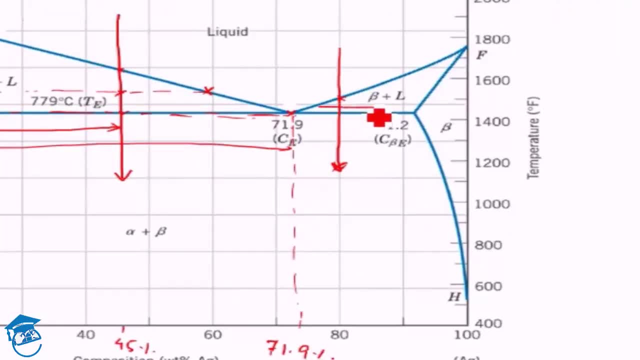 What would happen again? What would happen again Again is over here. the liquids composition would be this and the solid would be this: at eutectic temperature, Again, the liquids composition would hit the eutectic composition and the solid would be somewhere around here, composed. 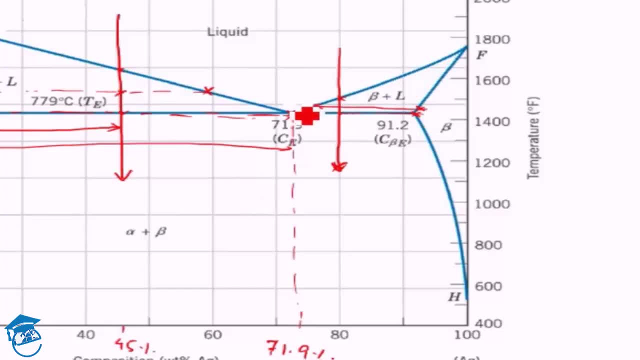 Thereby again, it does not matter whether you are at lower concentration or at higher concentration than the eutectic composition Upon relatively slow cooling, such that it equilibrium is maintained. as soon as you hit the eutectic temperature you will get. 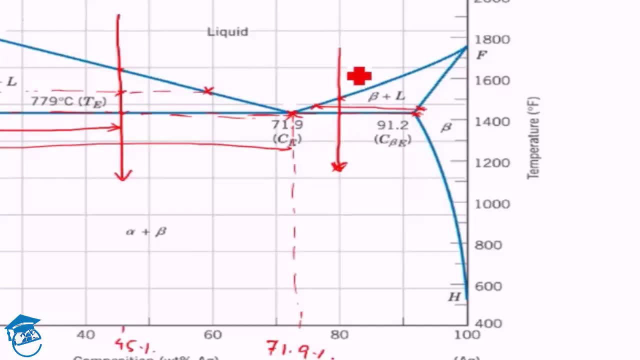 a liquid which is of eutectic composition. So what will happen in this case? In this case, you will get beta plus liquid in eutectic form which converts into alpha plus beta on further cooling. So this gives you an idea about the eutectic system. We know that eutectic 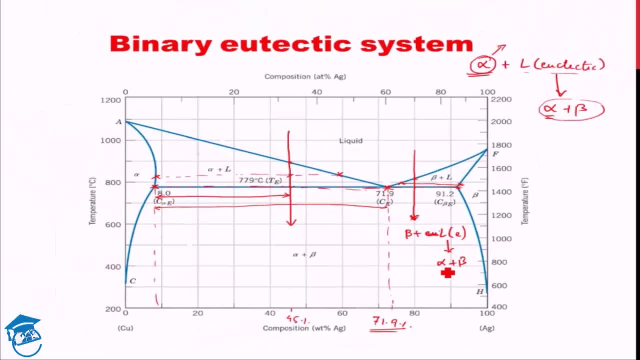 system is transformation of liquid into two solids simultaneously and we saw that the eutectic reaction. for the eutectic reaction to occur, we need not be at the eutectic composition to start with. Eventually we will get some amount of liquid which is at the eutectic. 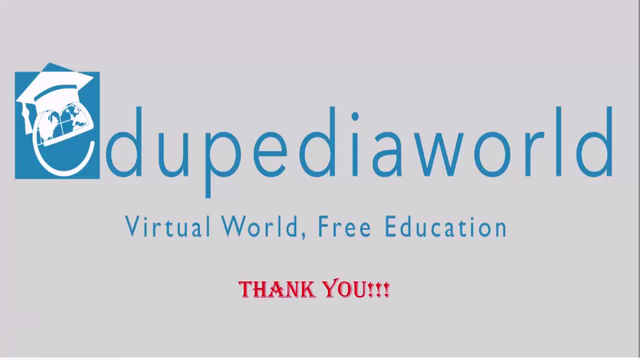 composition. With this I will conclude today's lecture. Next lecture we will further our knowledge on phases and phase diagrams. Till then, have a great day, Good bye.